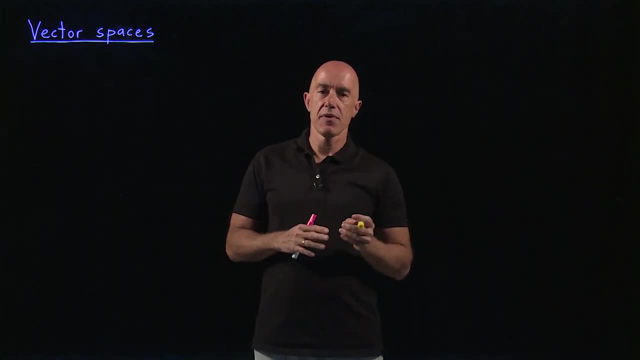 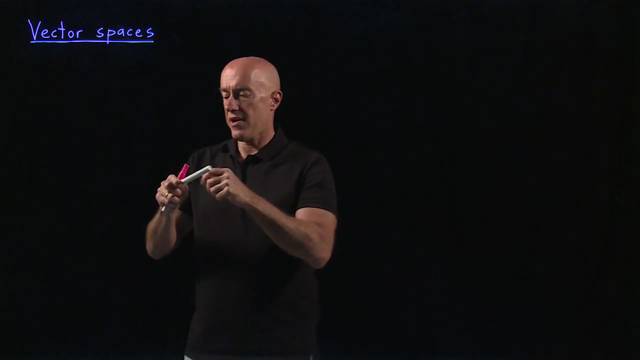 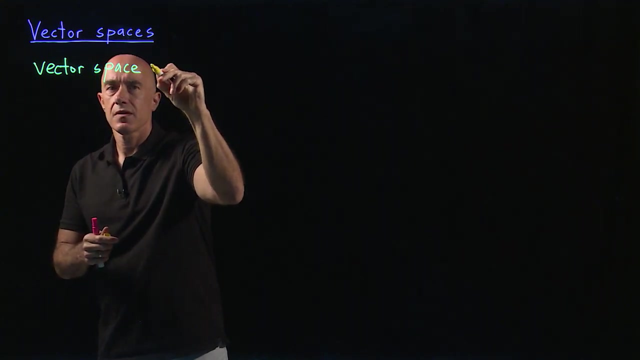 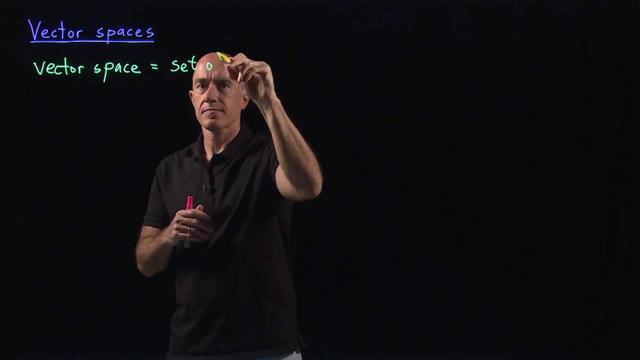 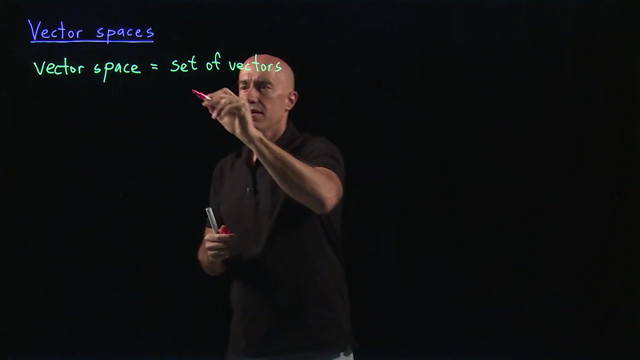 that are column matrices, But I want to be a little bit more general. so let's first define what a vector space is. So a vector space consists of two things. One is a set of vectors. In this course, the vector space will be simply column matrices. But, as I mentioned, vectors can be more general than just column. 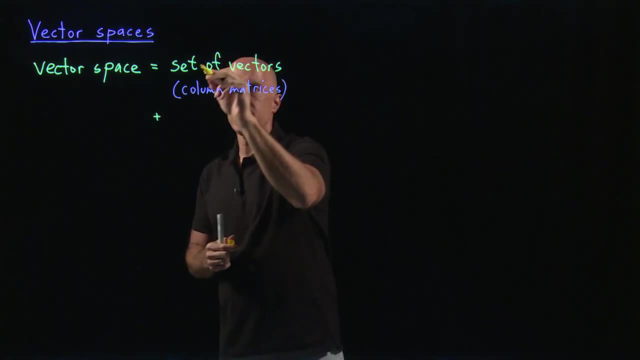 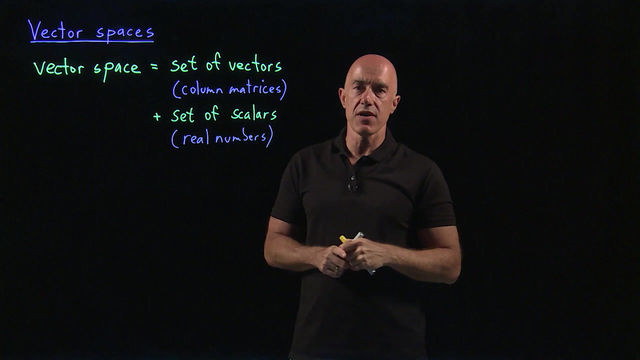 matrices, And in addition to the set of vectors, you need a set of scalars. In this course, the scalars will simply be the set of real numbers. Typically, the set of scalars can be also the set of complex numbers, but we won't deal. 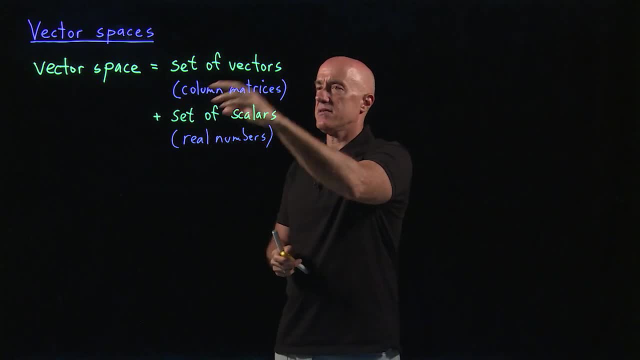 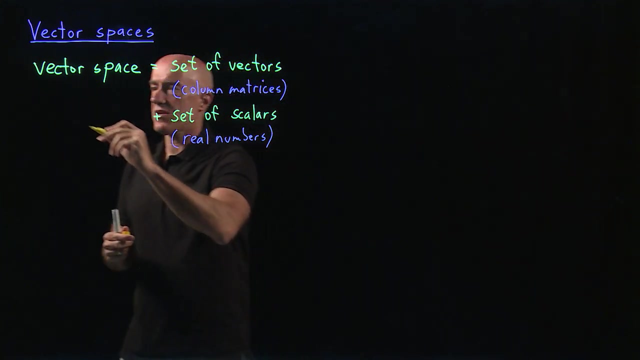 with that in this course. So a vector space consists of a set of vectors- could be an infinite set and is likely to be an infinite set- and a set of scalars, such as the real numbers, that has a certain property, which is that it's closed. Well, that's the case. 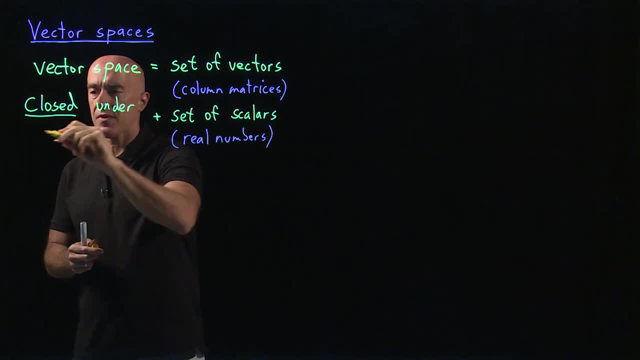 So what are the set of vectors? Well, the set of vectors are simply a set of numbers. They're what we call store, the sum of the inside and the outside. OK, So what does it mean that you can store the sum? Well, we're going to look at the vector space, the set of vectors. 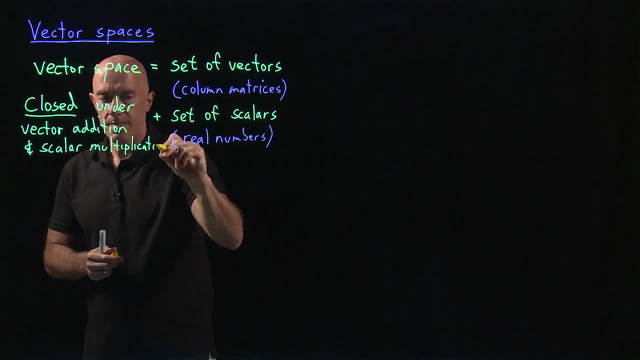 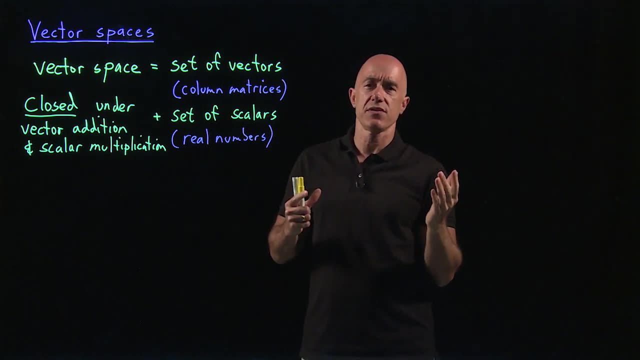 just right here. where is the key and what is the key? Closed under vector addition and scalar multiplication. OK, What's the meaning of closed? It means that if you have two vectors in your vector space and you multiply them by scale, you can store them, but they're not the same thing, So you 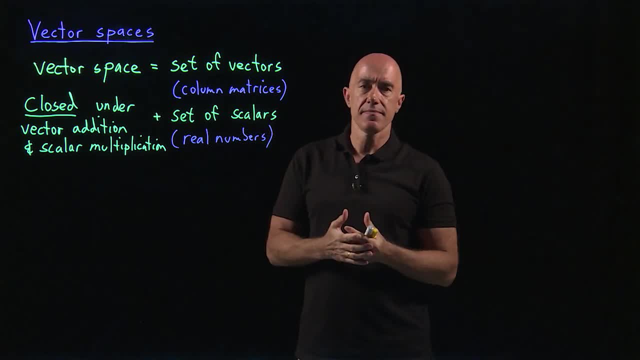 might have to find a way tochen them and store them, And also the fact is that people are just playing with the key for a certain reason, But I don't know if that's the right thing. but you scalars and then add them. The final result is also a vector and it has to be a member of your. 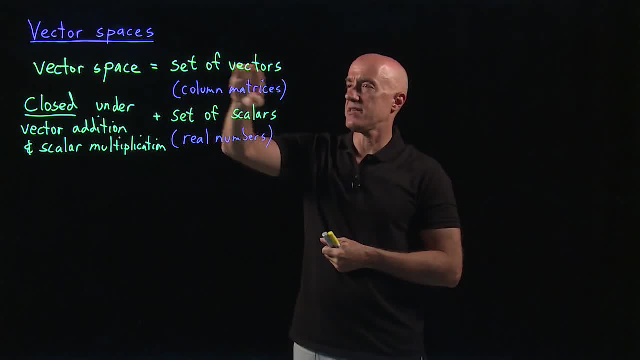 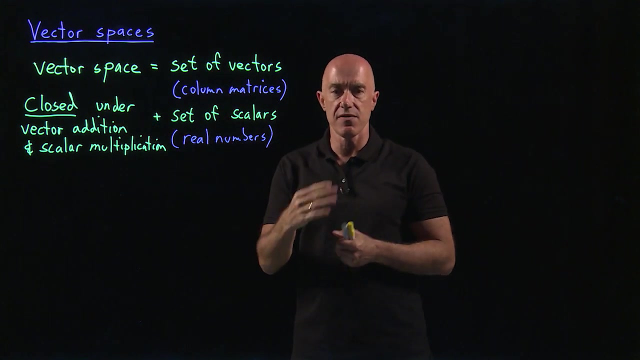 vector space. So, starting with a set of vectors that form your vector space, you can multiply them by scalars and add them, and you don't leave that set of vectors. You stay in that set of vectors. That's the meaning of closed. So we can look at an example of that. So what is an example? 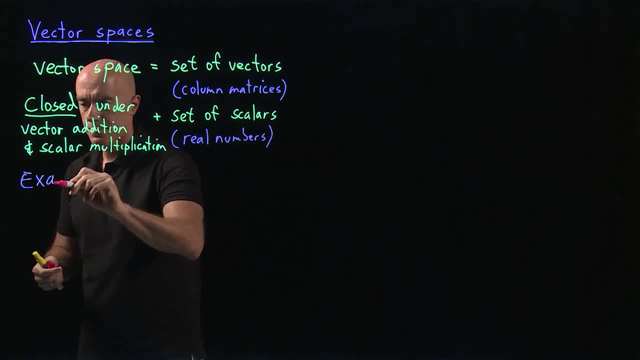 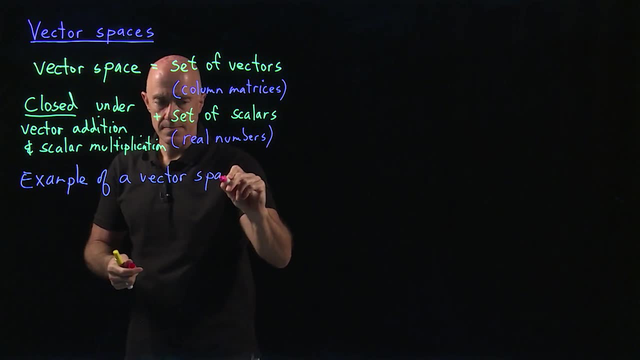 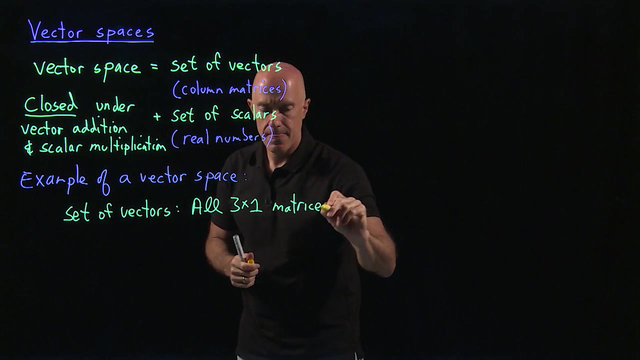 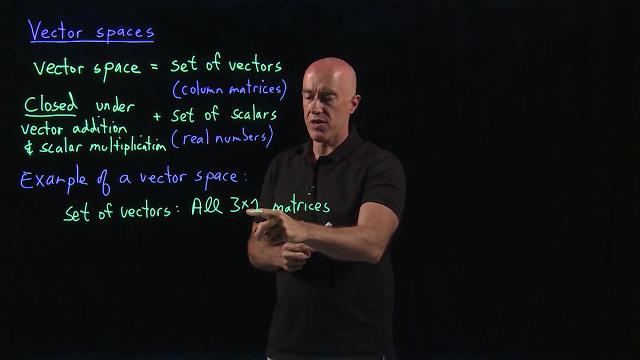 of a vector space. So we need a set of vectors and a set of scalars. So the set of vectors will be all three by one matrices. right, Those are what we called column vectors before, or column matrices, So they have three rows and one column. So that's our set of vectors and the set of. 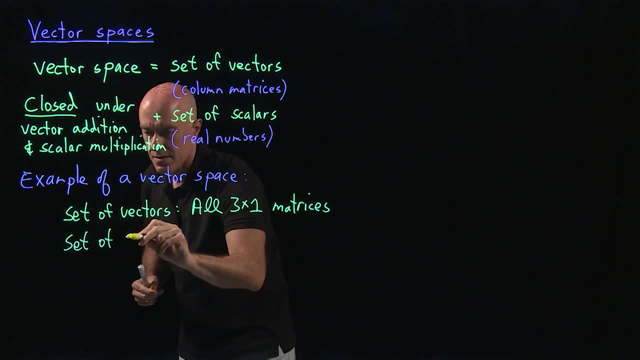 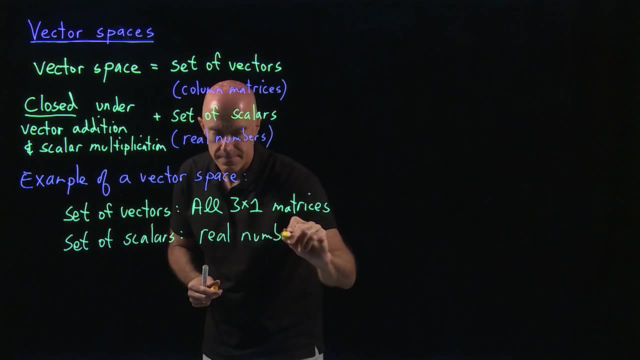 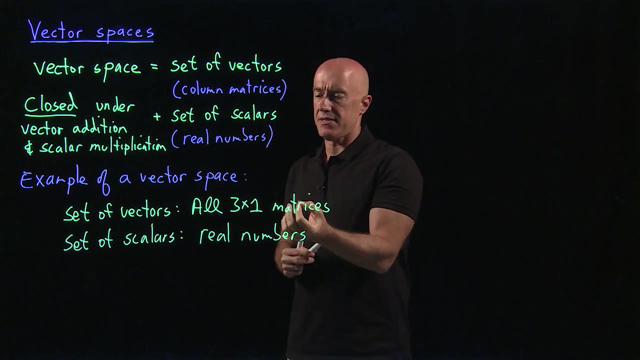 scalars are just the real numbers, Right? I claim that that's a vector space. My claim that this is a vector space means that if we take any three by one matrix, multiply it by a real number and add it to any other three by one, 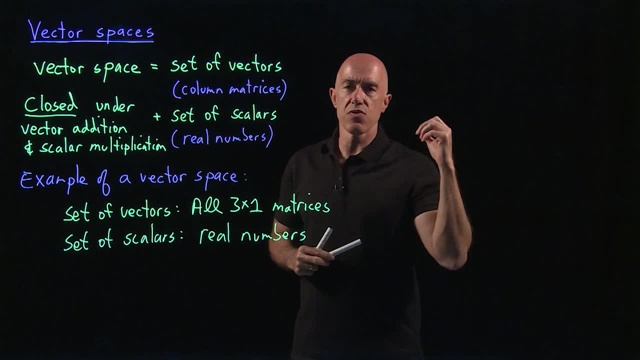 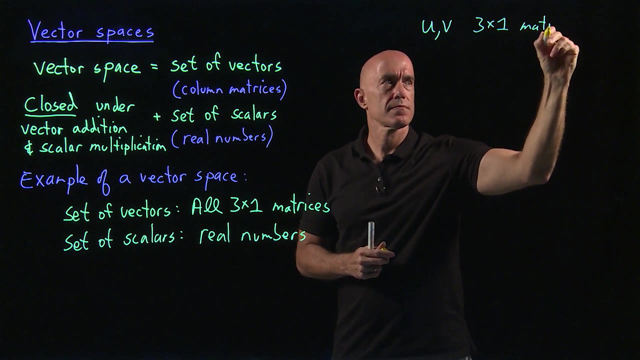 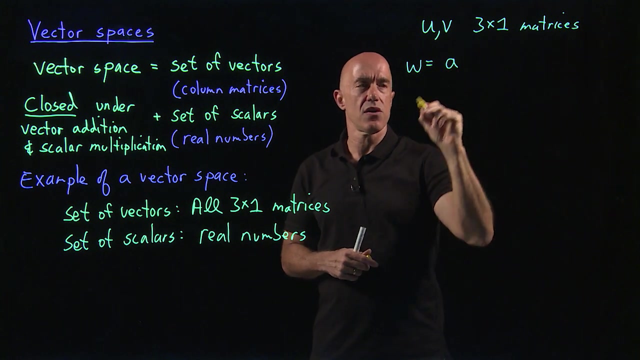 matrix. multiply that by a real number, do we end up with a three by one matrix. We do right. So in this case u and v are three by one matrices And we take w equals a scalar, a real number times u plus a real. 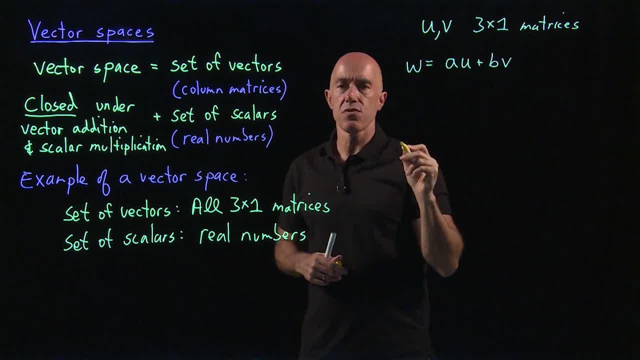 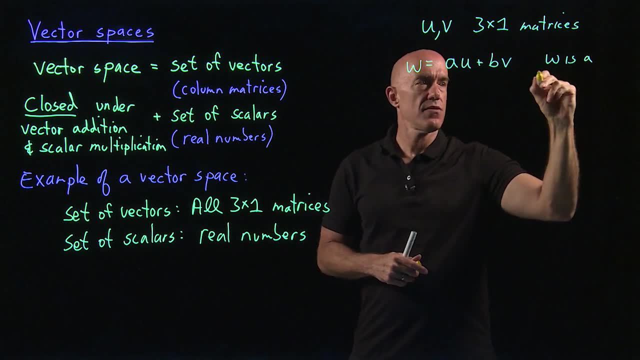 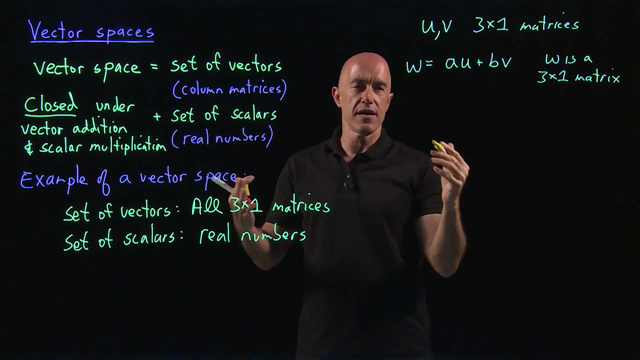 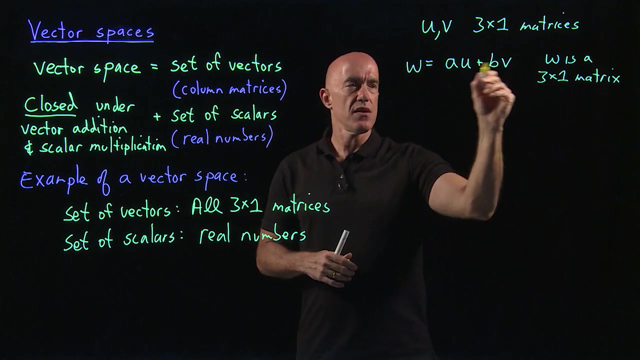 number times v, Then is w a three by one matrix. Yes, right, So w is a three by one matrix. Okay, We can illustrate that as explicit as you want, right? So that's basically saying: if we have a times a three by one matrix- x, one x, two x three right plus b times another three by one matrix. 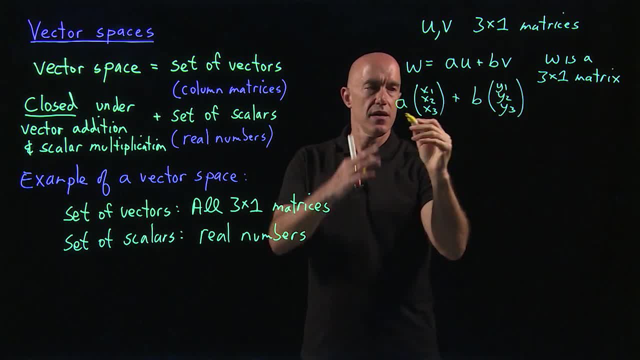 y one, y two, y three. If we do this then A equals one thing, As you could see over here in this figure, the value of the four- think a x times b- equals first If we multiply all three of these.